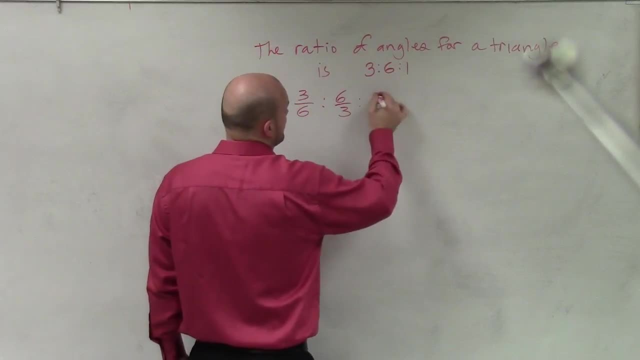 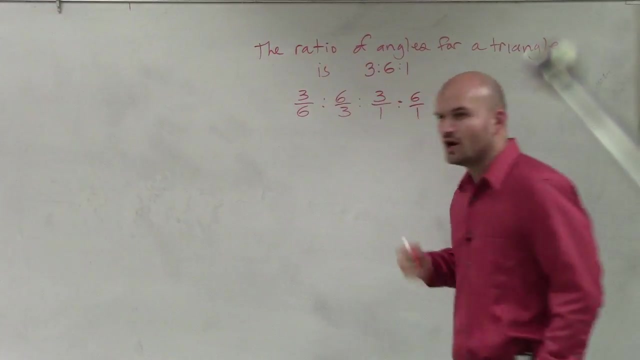 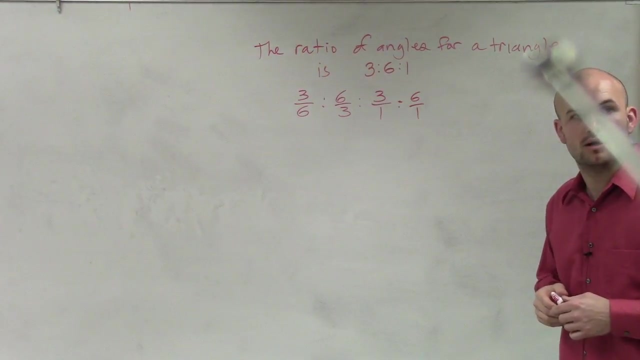 six is to three, three to one, six to one. They're all comparison to each other. These are all angles that are in the comparison, right? So all these angles are comparing. you know, we're all comparing each other, But remember, these are all angles. 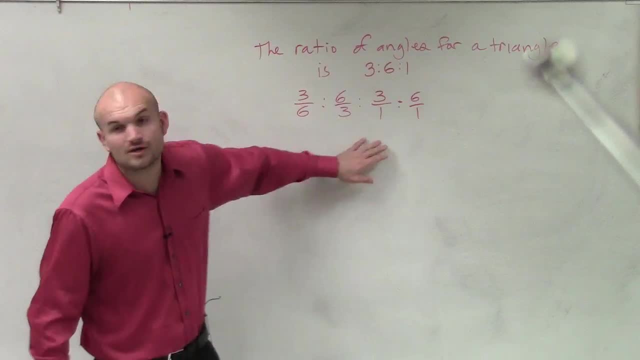 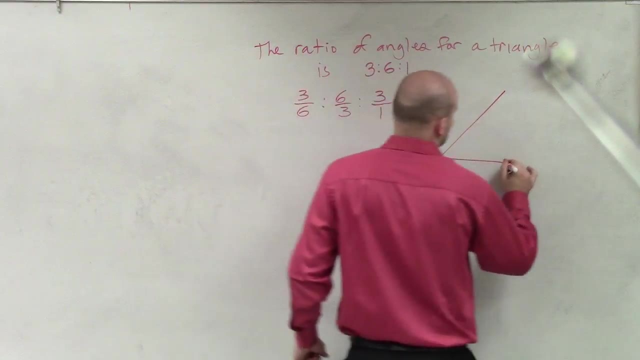 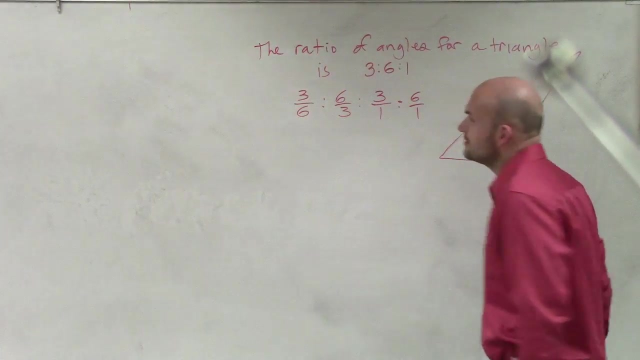 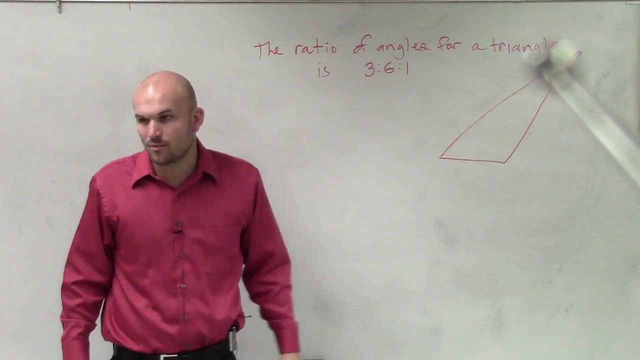 These are all angles that are comparing within the triangle. all right, So what we're going to do is obviously, guys, if you look at this triangle, we know that angles cannot be three, six and one. right, We know that's not true, right? The same thing If I said: 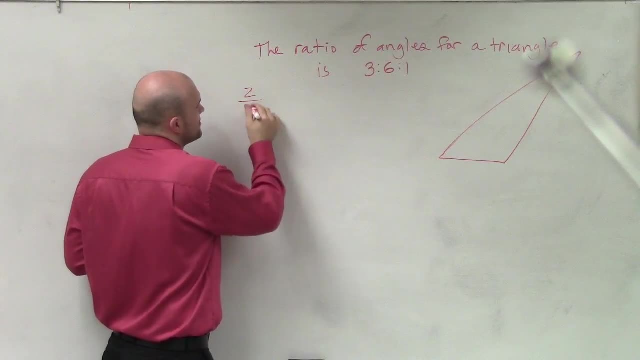 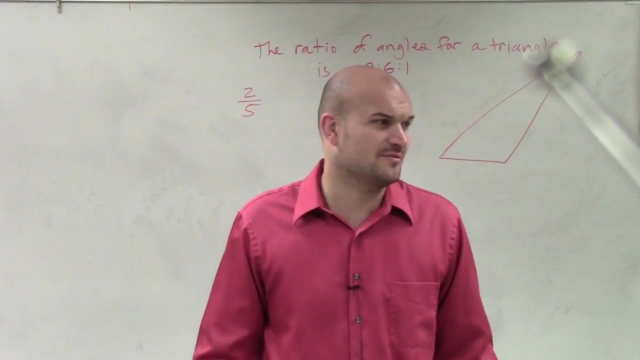 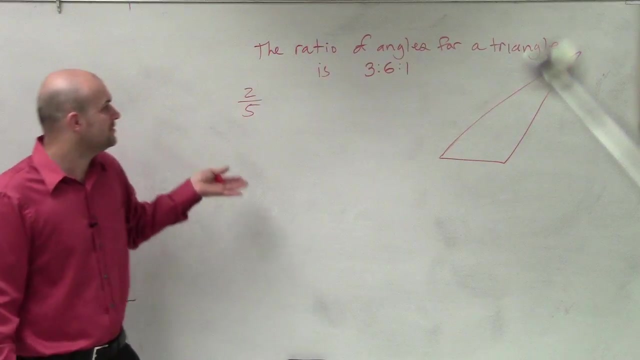 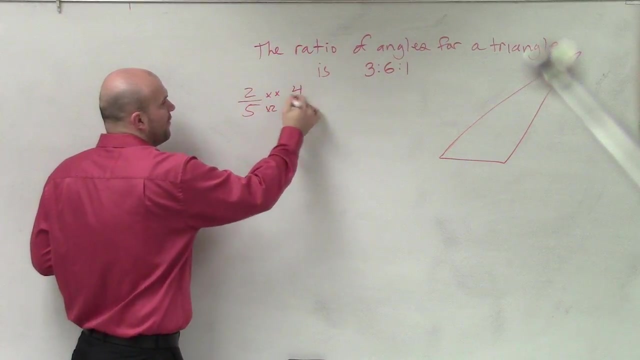 let's say, there's two girls compared to five boys in this classroom. Well, is that correct? No, there's not seven people in this classroom, right? That's the reduced fraction, right? So, and if we say, well, there's 10, you know, there's actually 14 people in this class. what you do is: you know, really, when you multiply by two over two, you get four over 10.. In reality, there's four girls and there's 10 boys, right? 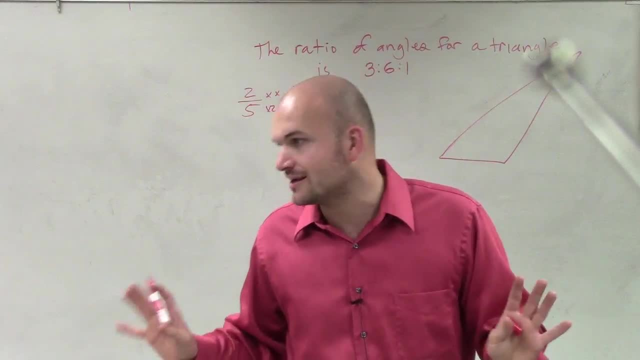 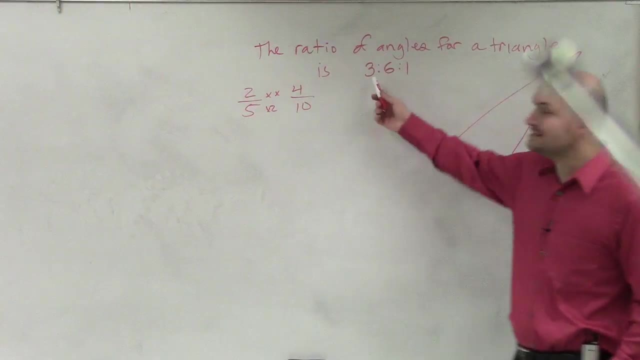 but a lot of times we use. there's not really that case at all. look around, But what we use is we reduce. when we're doing ratios, we reduce it, all right. So what I need to do for this is I need to say: well, what, how much did I reduce this Right? am I multiplying by these by two? So when I say the angles are six, twelve and two degrees, Do I multiplying by two? Does that make sense for the angles of a triangle? 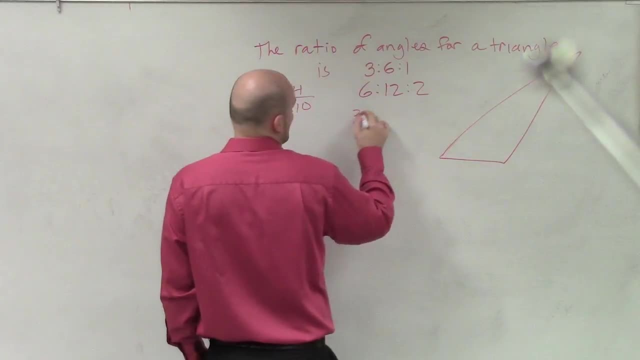 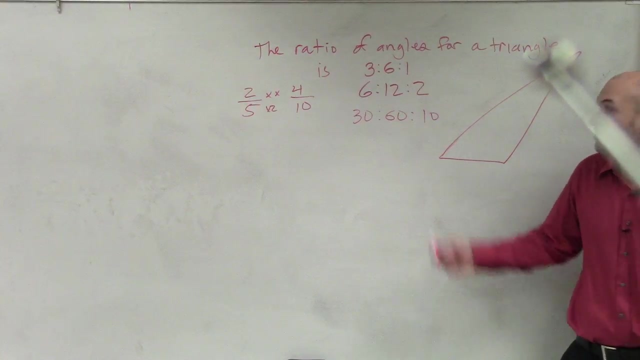 No, Do I multiply it 10 times 30,, 60,, 10?? Can that be the angles of a triangle? No, But remember, all these all reduce down to 3,, 6,, 1.. So what I need to do is say: well, how much am I? 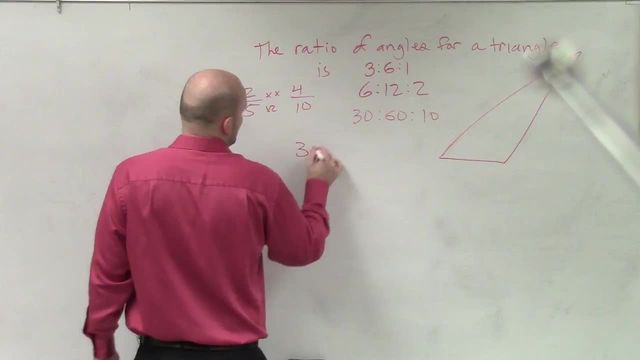 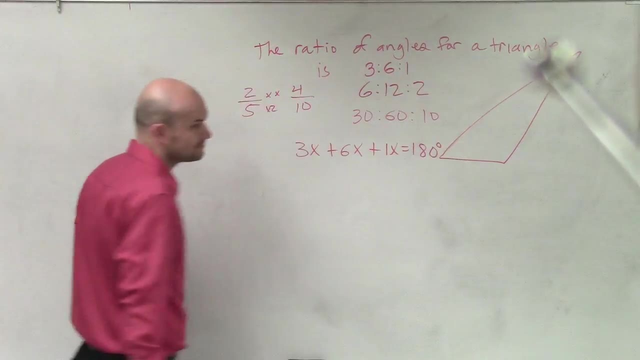 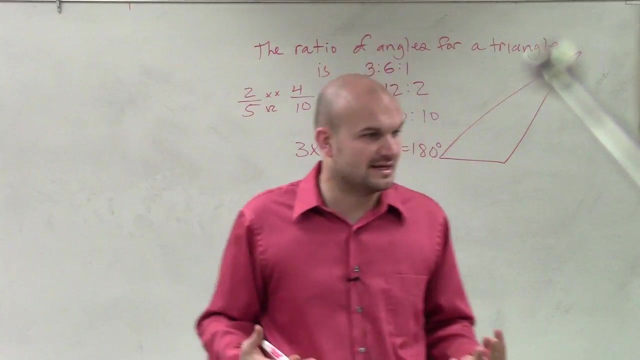 reducing it by. So what I do is I create a triangle- 3x plus 6x plus 1x equals 180 degrees, And I do that to help me now determine our value of x. where x tells you what are you reducing?